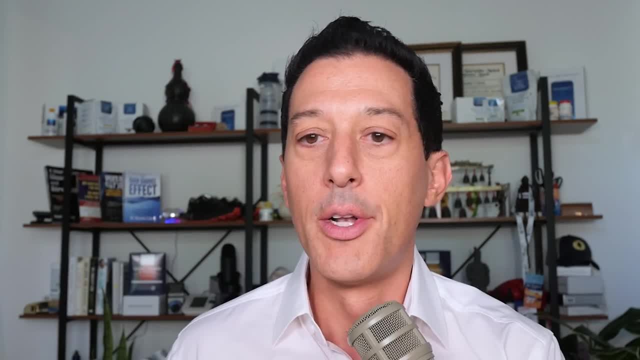 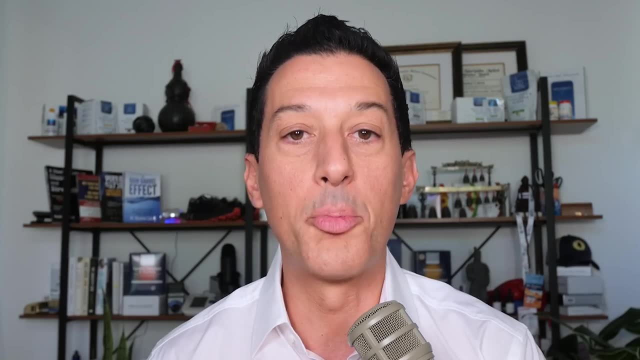 most pervasive in the environment, simply because it's in our tap water. antiperspirants, a lot of cosmetics, It is in shots as well. It is all over the place, right? It's your cooking pans, spatulas, et cetera. So when you scrape those pans or you, 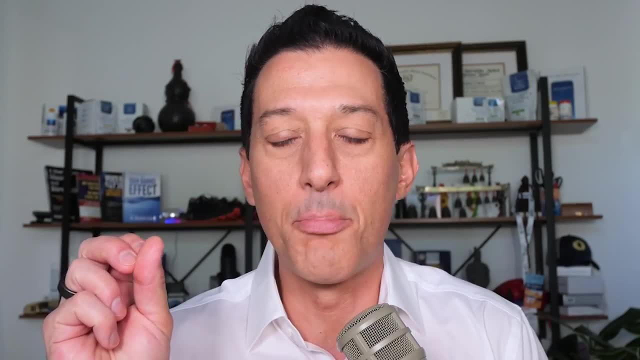 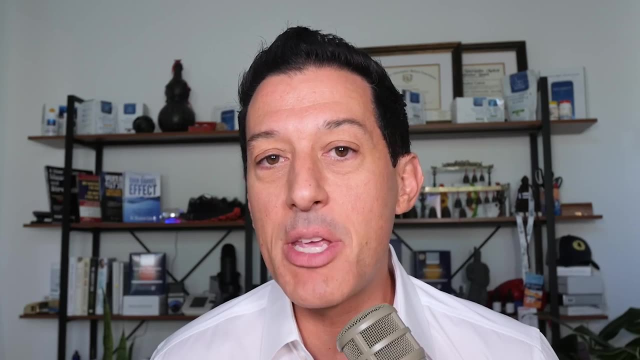 use aluminum foil, you get a little bit. And these are micros, right, Little micro particles in the body, but they add up over time. They really do. They add up over time. That's the issue with them. All right, We've got cadmium. That's another one That can be in cosmetics. That can be in 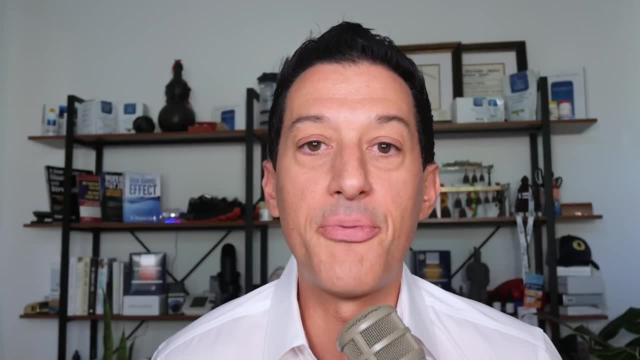 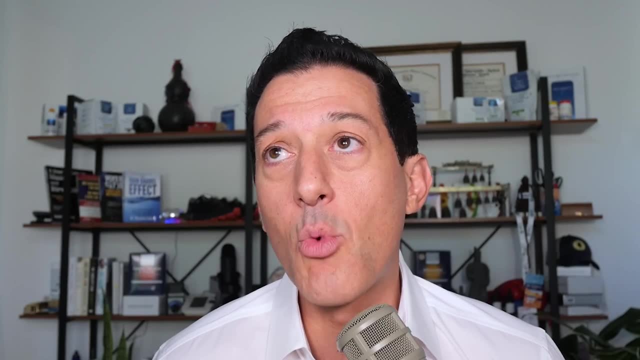 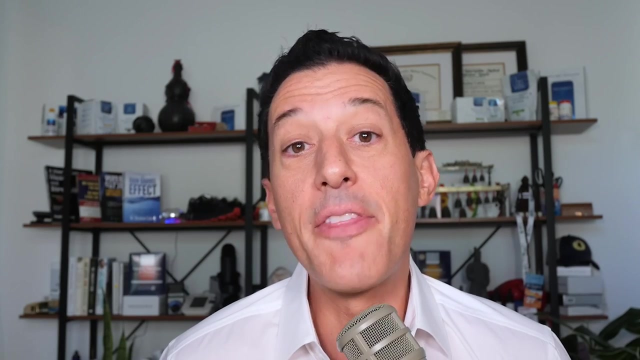 batteries. That can be in certain machinery. Cadmium can also be found in certain foods, So it's another one that we watch for. Arsenic: pretty pervasive in water. It can be in groundwater too, So in gardens or anything growing in groundwater. rice is the most named one for arsenic, And then 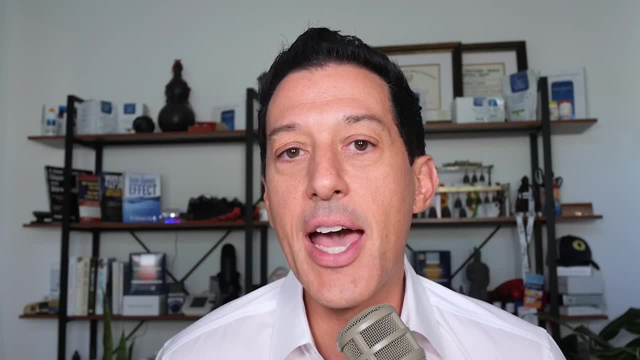 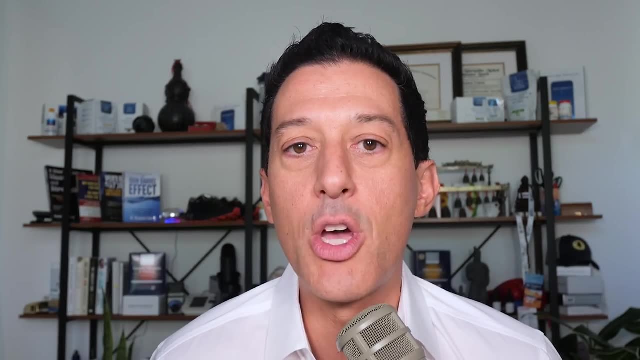 we have lead, And so lead is a huge one. We'd be careful of that. Many homes- older homes or older cities- still have lead pipes, But lead could be in multiple things: Lead paint- we know older homes, et cetera. 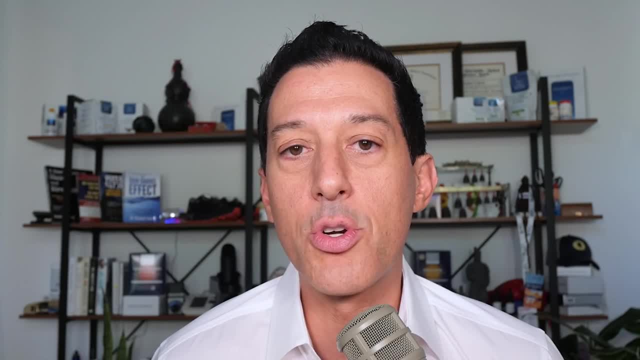 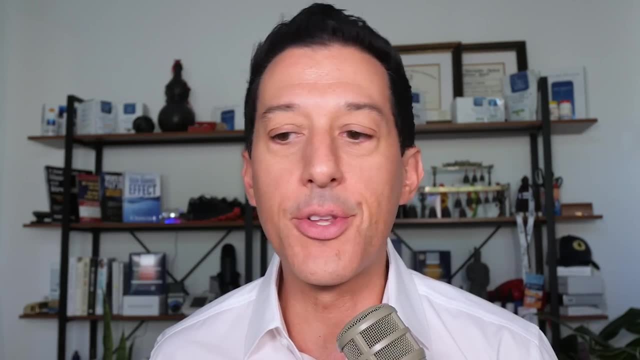 So the problem is again: a lot of these times or a lot of these exposures are just in micro particles, but they add up over time And if our body begins to accumulate them, they end up in our organs. So they end up in liver, kidneys, spleen et cetera, And they can. 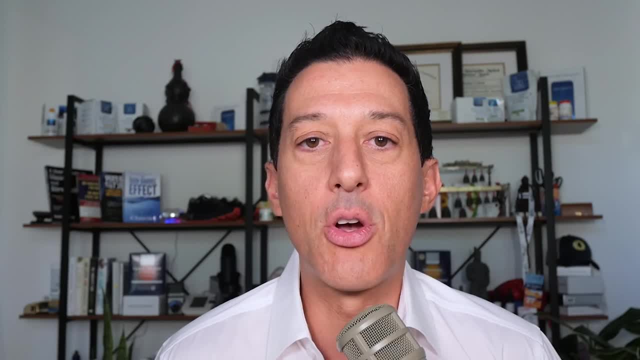 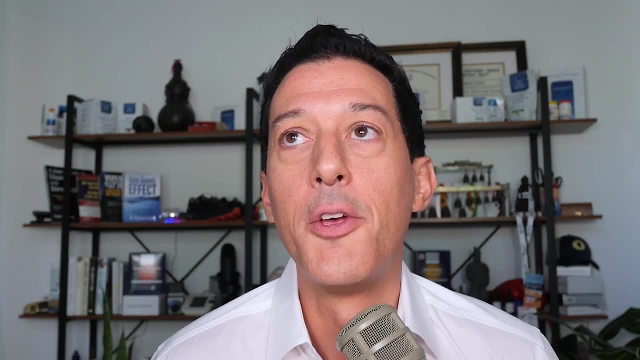 also end up in the brain, potentially causing things like dementia, Alzheimer's and the nervous system with Parkinson's, et cetera. That's why it is important. I mean it really is. We don't always want to look at just the end goal because, sure, if you have heavy metal poisoning, you're 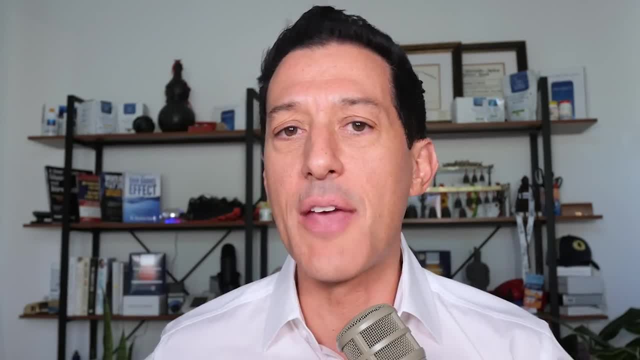 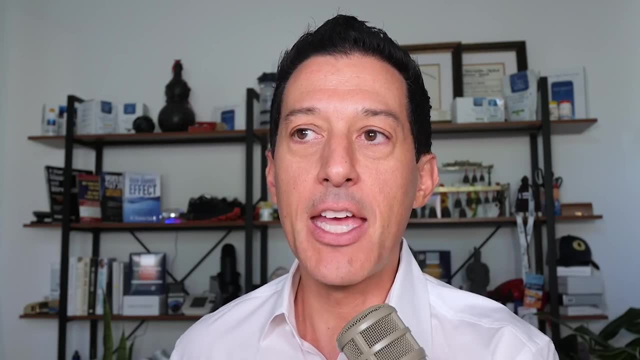 looking at fever, vomiting, nausea, et cetera. We're not talking about heavy metal poisoning, So that's not what today's show is about. Today's about chronic illness, chronic dis-ease in the body, And conventional medicine still is. 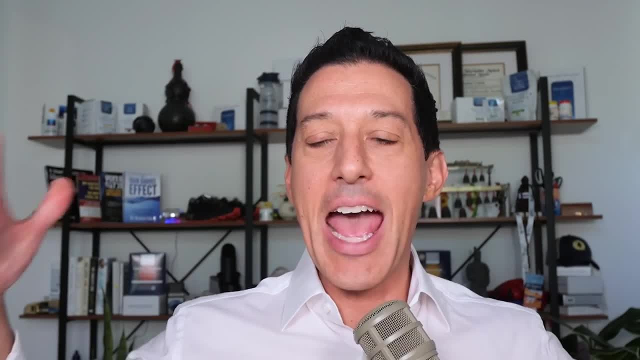 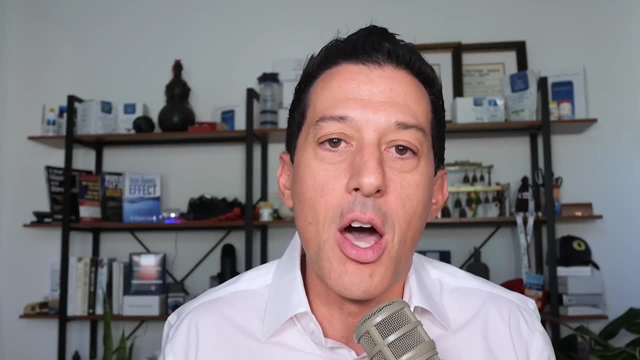 not understanding disease pathology. I mean, they know how these things happen, but they don't look at it. It's basically for them it goes from A to Z. So one day you didn't have cancer, the next day you did. Well, I mean, there's obviously something in between the two right, One day you 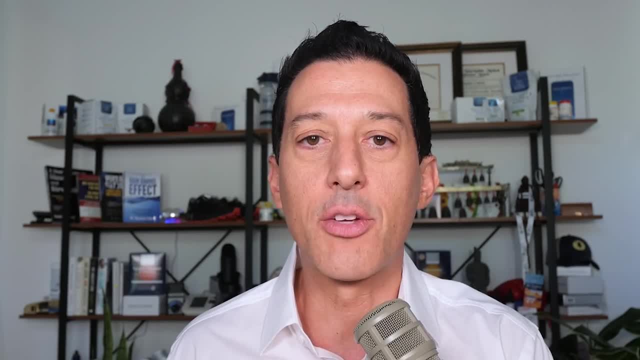 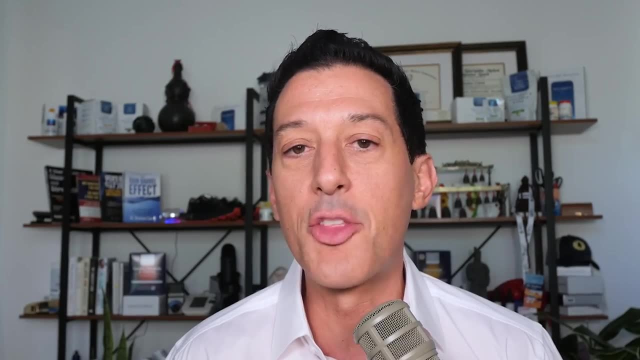 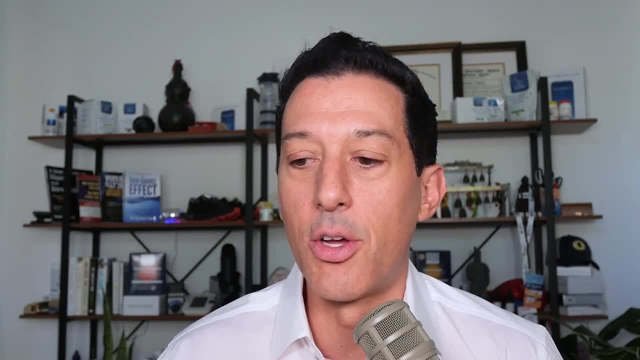 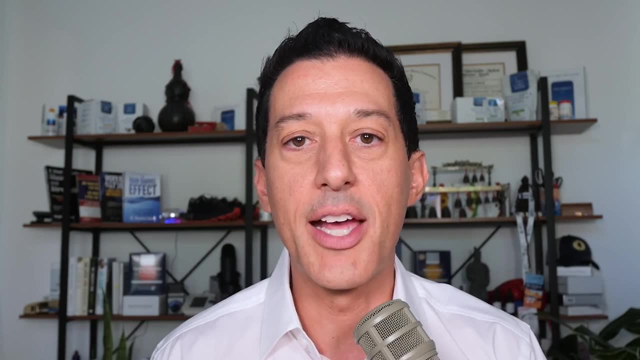 works? Not even close. We know that Alzheimer's- they thought that Alzheimer's just came about. Well, Alzheimer's has created decades before, And what I want to do is just give you the early warning signs. These are the things to look for because they can be overcome, They can be fixed. 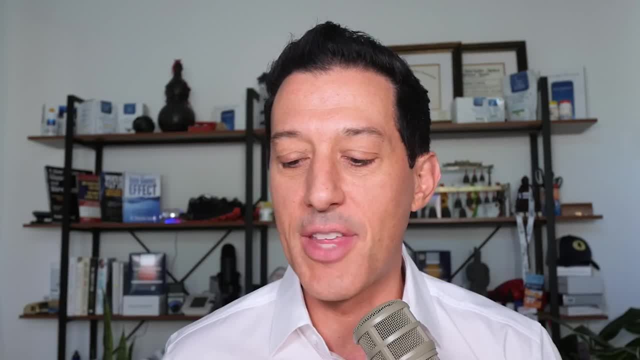 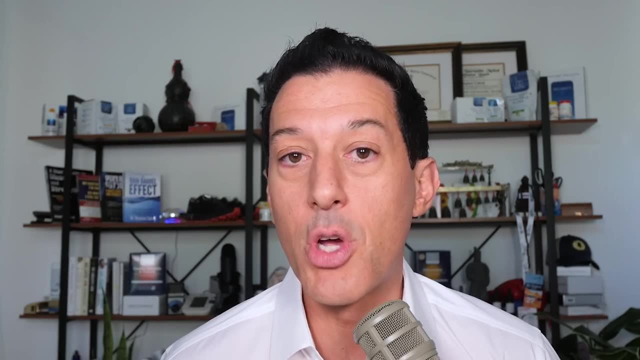 So I would never give you anything just to scare you. I don't believe that that's what anybody should be doing. You should be knowing and understanding that there's always an answer. These are the underlying root causes that we're talking about. Not difficult to rebalance the body, Typically six to 12 weeks- That's all that it takes for. 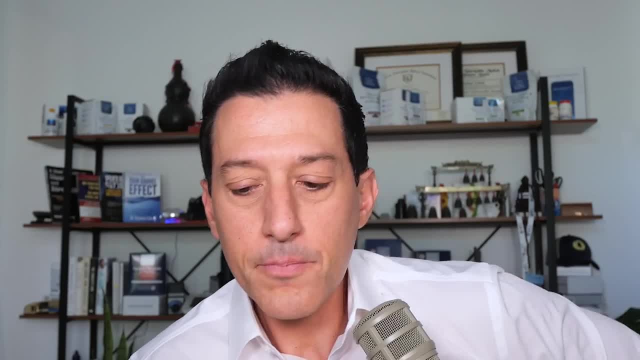 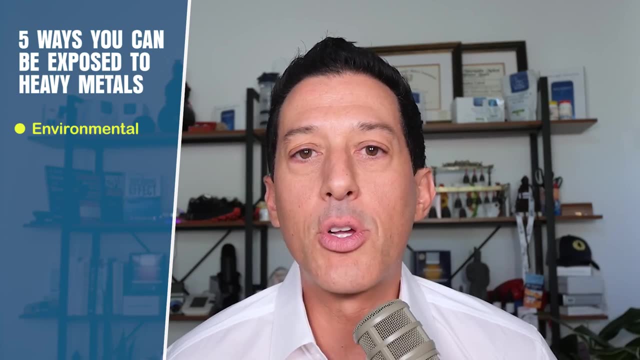 most people. Honestly, that's the truth. Okay, let's get into the five main ways people are exposed. The first one's, environmental. I might do a whole show on this specifically, but for right now, environmental water pollution. it's the truth. Pesticide sprays on our food and our lawns. 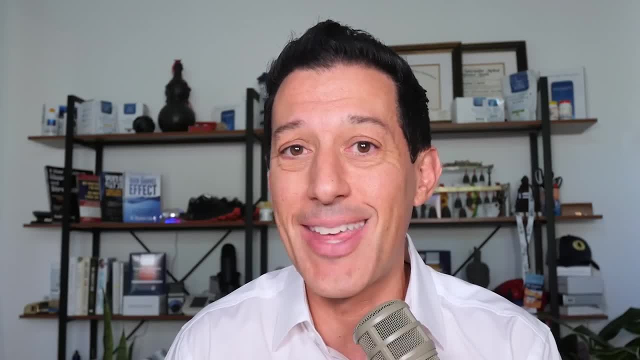 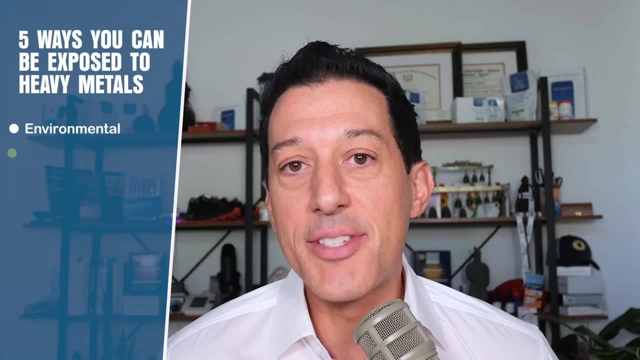 which can have heavy metals in them. Not as much, but they absolutely can. I mean, even some organic pesticides have high levels of copper in them. Ports, pots and pans that I spoke about before can have high levels of aluminum, And again, 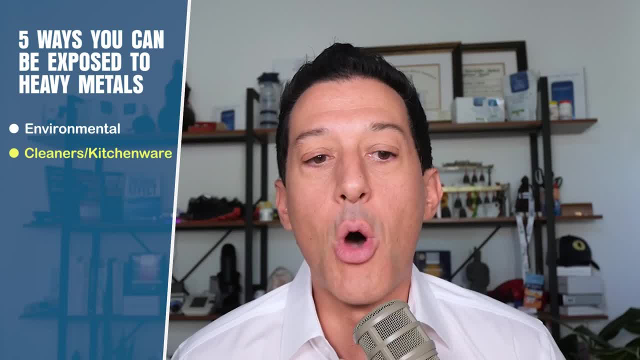 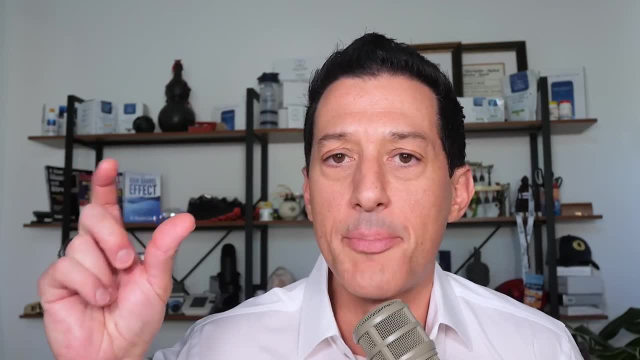 aluminum foil. We'll talk about that actually in just bath products. So occupations: we do environmental testing for people all the time, Simple urine-based test. If you're interested in any of the at-home lab tests, you can find them all at stephencabralcom forward slash labs. 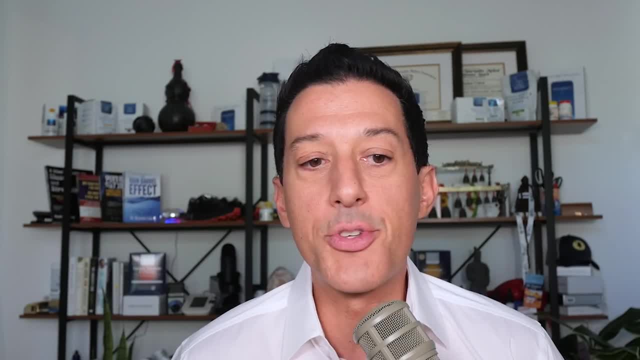 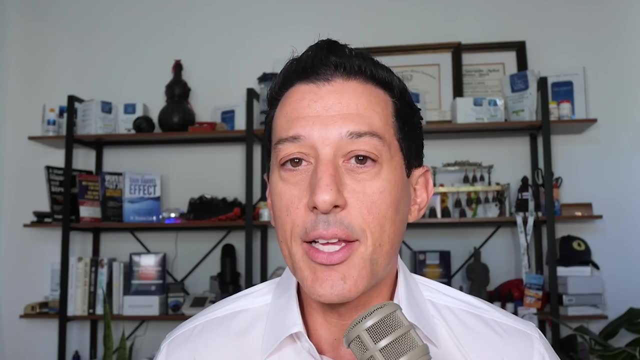 Feel free to check them out Again. no obligation to run any of them And, of course, you don't have to run them with us. You can run them with your local naturopathic doctor or integrative health practitioner, Mechanics, nail salons, hair salons, dentist's office- a lot of places where these heavy metals 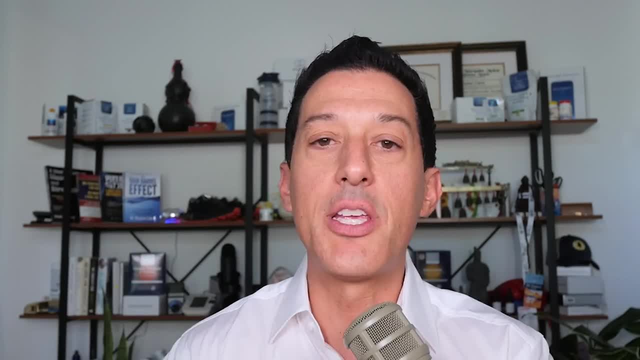 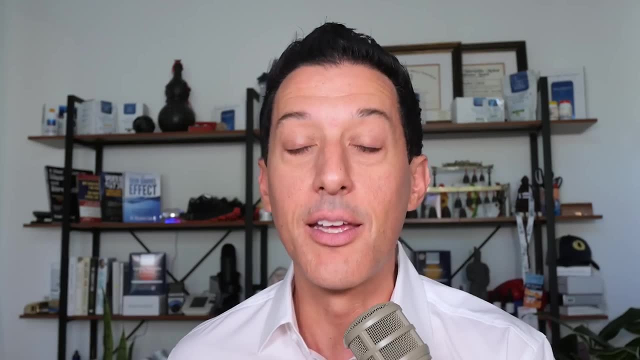 can show up. Okay. so again, if you're working there at one of these places, I want you to make sure that you're especially careful. But the other part is is that if you attend or you're at any of these places, quite often it can affect you as well. Just in the air these things are vaporized. 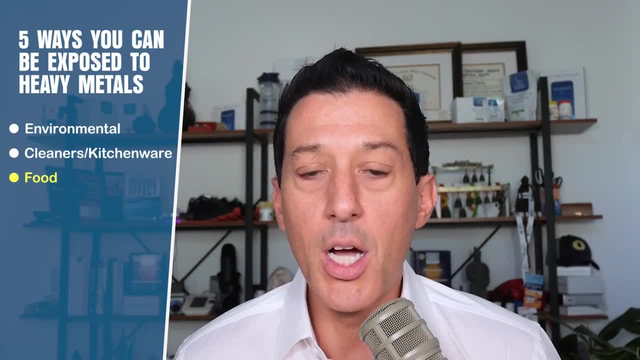 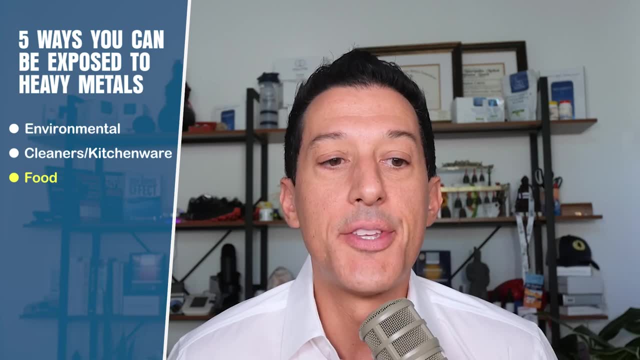 as well. All right for food, processed food fish. So there are fish that are higher in mercury. I will link to that in the description. I will link up a podcast to share that one with you. stephencabralcom forward slash 2575.. 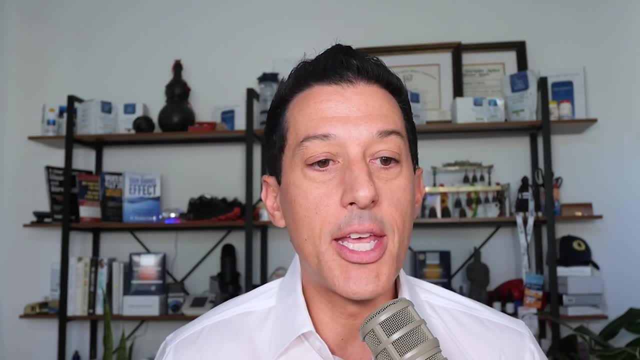 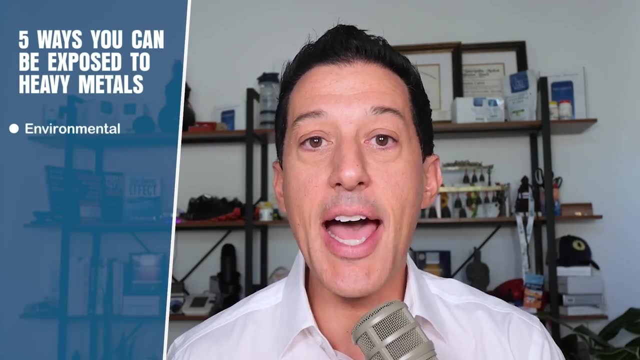 We want to look at rice, making sure that rice is not containing arsenic. A lot of processed foods contain things like bromine, but they can also contain cadmium as well. Certain medicines- I cannot give you the scope of all of the medicine that contains heavy metals in them. Maybe I'll do. 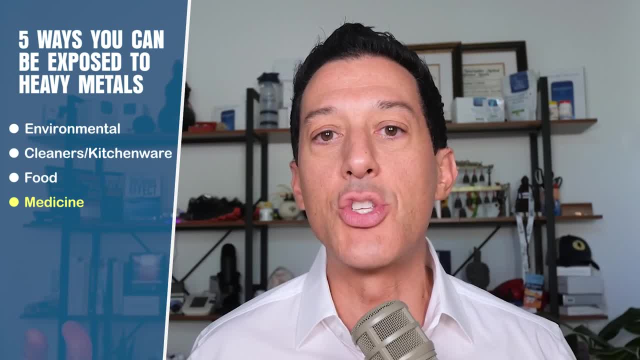 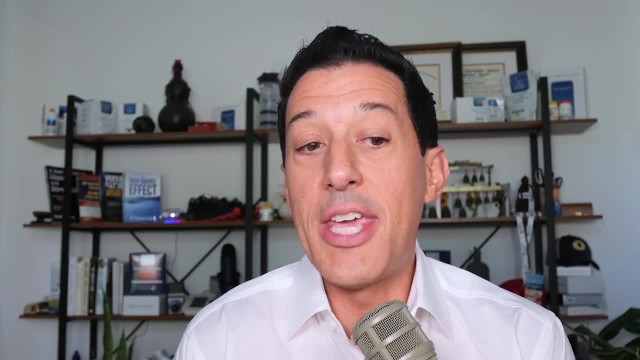 a specific show on that, Because if I gave you the list of medications right now, first of all, it'll be quite long, But the second is there are new medications being created, particularly every week. So what you can do, and I want to recommend this for you- 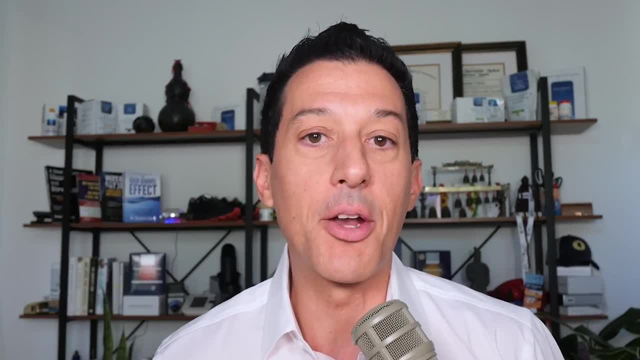 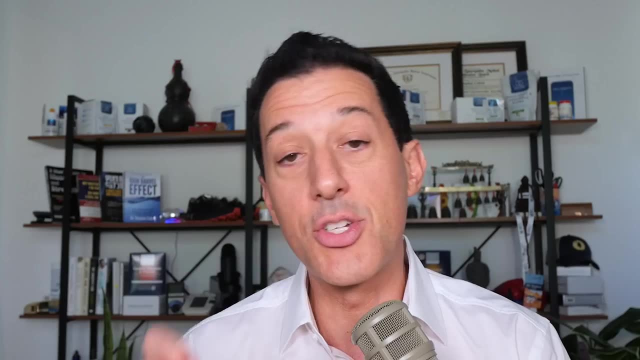 is that you type in your medication and you just say heavy metals. So like: are there heavy metals in statins? Are there heavy metals in your thyroid medication? And I think you'd be surprised. But you're going to find things like fluoride etc. And that these can. 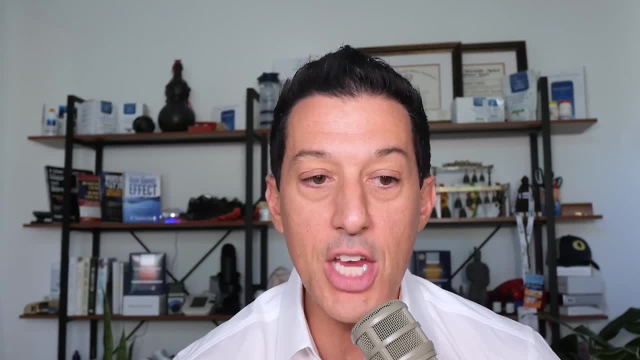 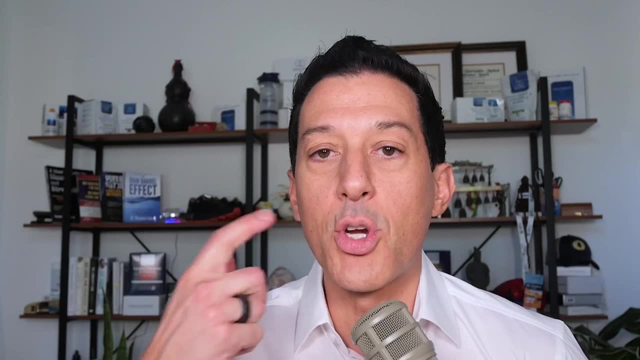 be quite dangerous. So also inside of medications there's that part, there's the shots that I've been talking about. There's also joint replacements- I know it's not a medication, but it's a medication- And mercury amalgams- the silver fillings inside your teeth- can have anything from nickel. 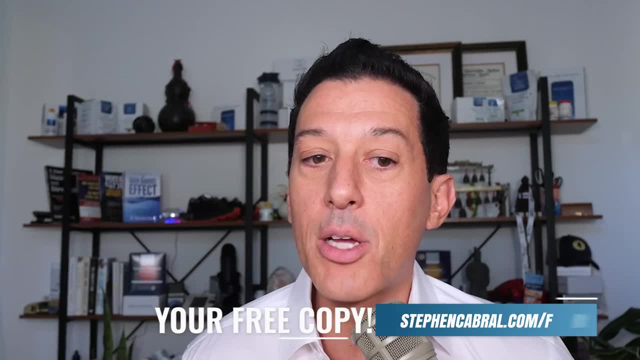 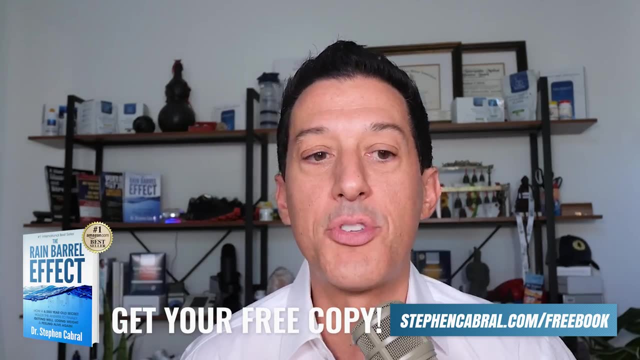 aluminum, mercury, etc. So if you haven't read the rain barrel effect yet, I would definitely recommend reading that before you might have those removed, because it's going to share with you the safest way to do that as well. And the last one is bath products- Deodorants contain 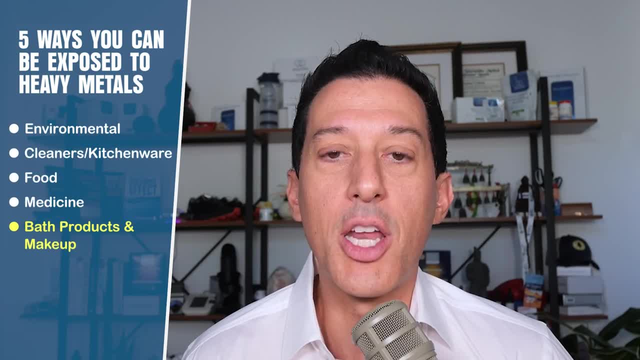 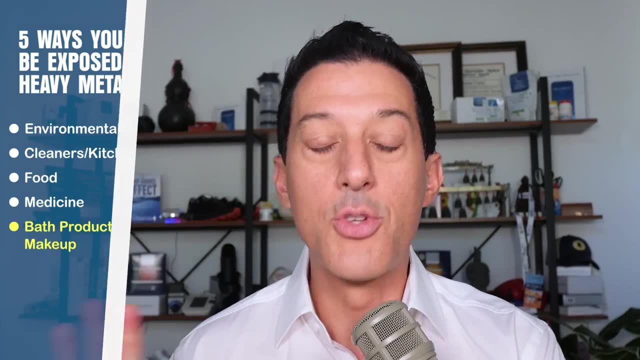 aluminum. I should say most antiperspirants contain aluminum. A lot of makeup does as well, So lots of shows on that. Again, all of this, this is in the rain barrel effect as well, So just making sure that you have those. So what I want to 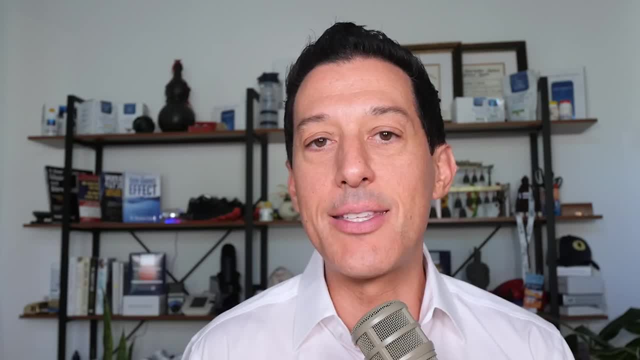 get to now, now that I give you a little bit of an intro, are the nine main symptoms, which is today's show. that's what that's all about of heavy metals, So I'll go a little bit into some. most we've been 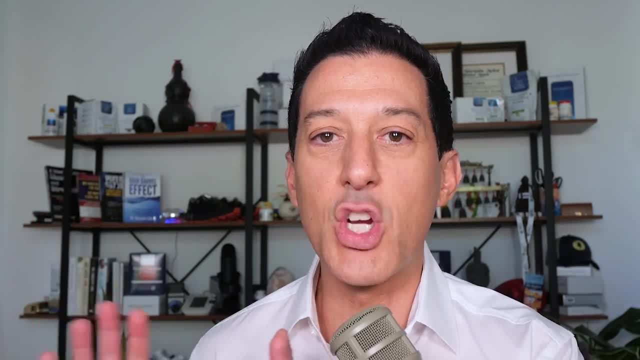 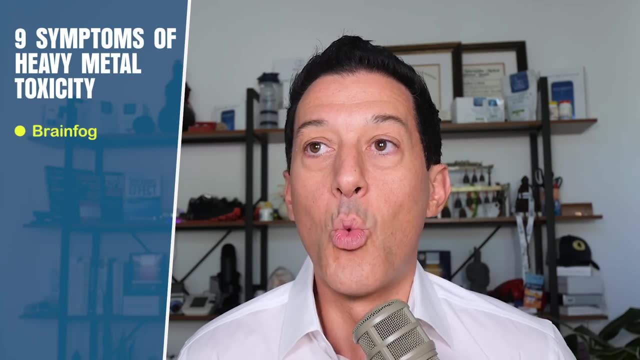 talking about on the show before, but I just want to make sure you can use this as kind of a quiz for yourself if you decide not to do heavy metal lab testing. Okay, so brain fog is a big one Whenever. well, let's take one step back. Heavy metals create inflammation. 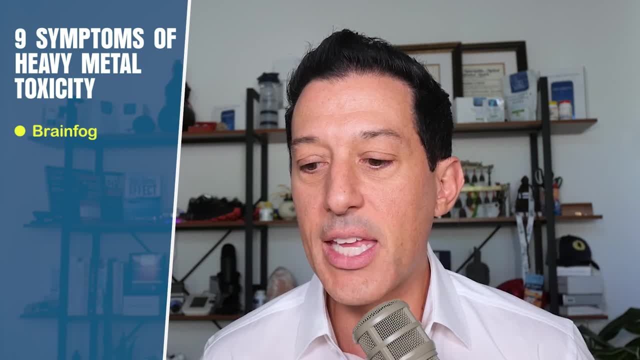 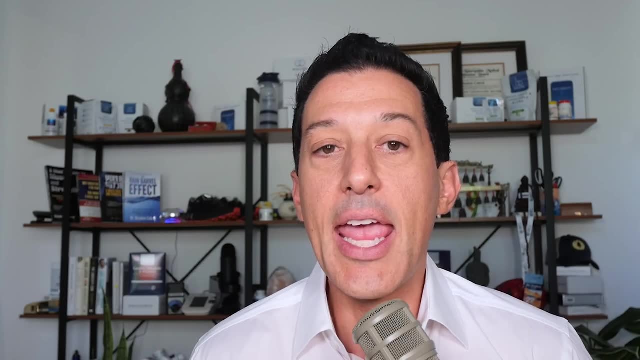 Heavy metals can end up in your digestive tract. They can end up in your organs. We talked a little bit about your spleen, your liver, your kidneys, your brain as well- And so what I want you to understand is: whenever there's inflammation, and there's inflammation in a specific area- 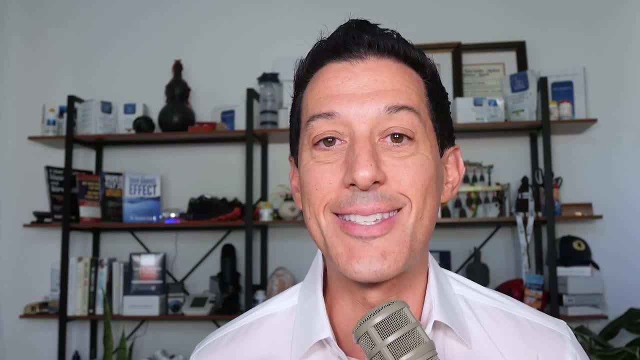 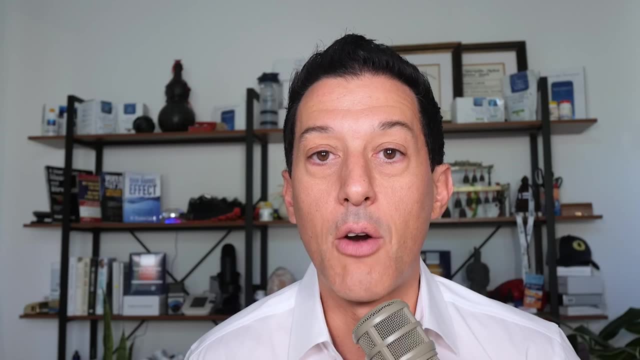 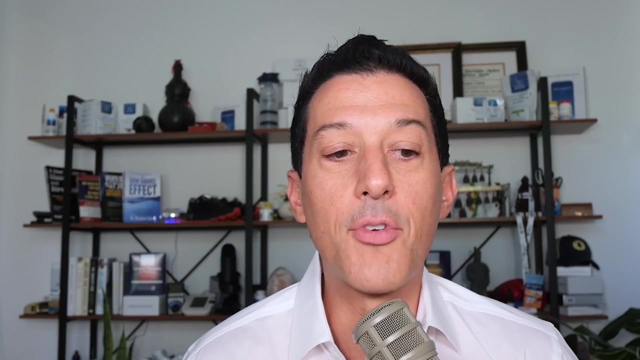 it can affect that area of the body or systemically. So inflammation in the brain, yes, but also just with the overall nervous system, is going to cause brain fog, All right. So inflammation also affects the mitochondria, causing inflammation Fatigue as well. So a lot of people with heavy metals have really bad fatigue. So I had Addison's. 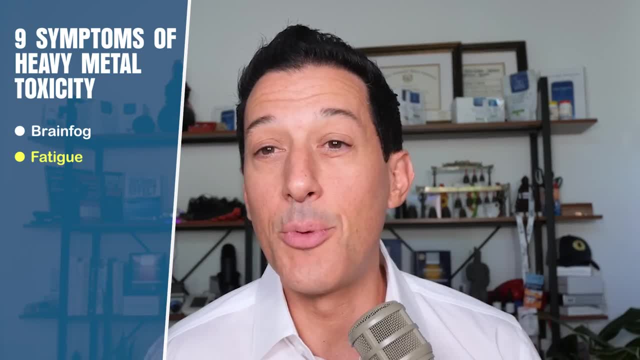 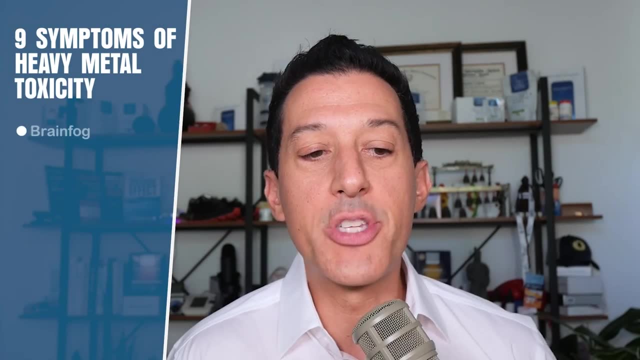 disease, but chronic fatigue, myalgic encephalomyelitis. I can tell you I had lots of mercury. I had high, high levels of mercury. I had to detox those before I could really get well. Many people it shows up as anxiety and depression or exacerbation of PTSD. So tics or anxiety. 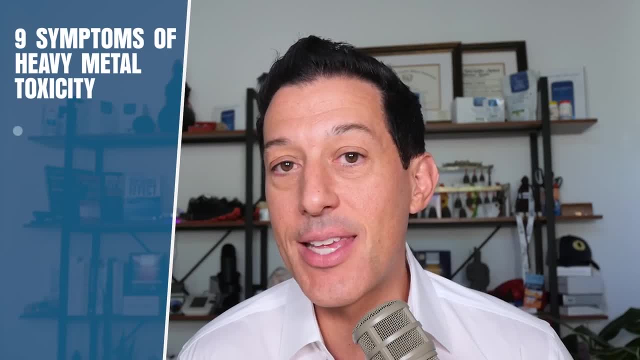 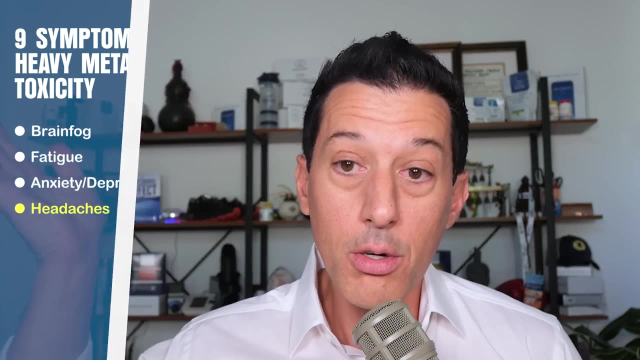 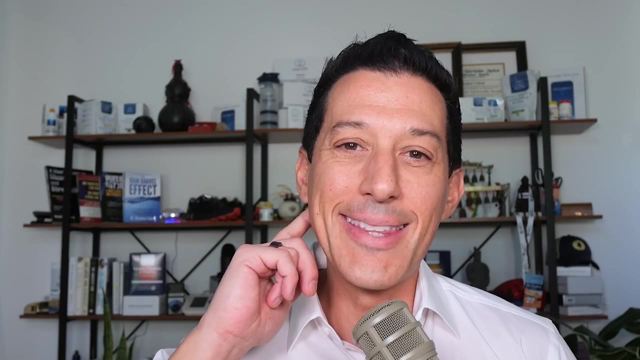 depression really prevalent Headaches. migraines is another big one, because all it takes is just a little extra inflammation. You start to constrict the blood flow, or increased blood flow, typically not the case up to what's called the trigeminal area. It's the area on the neck, right behind the ear, that can cause headaches. 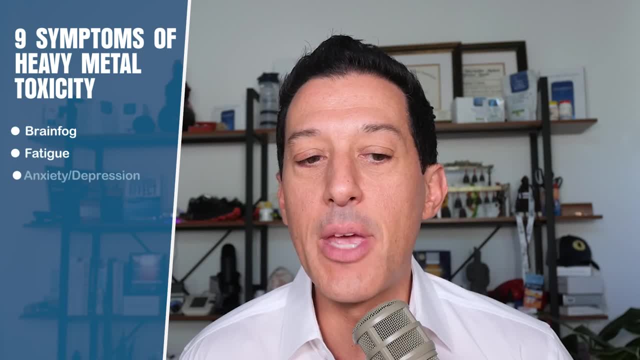 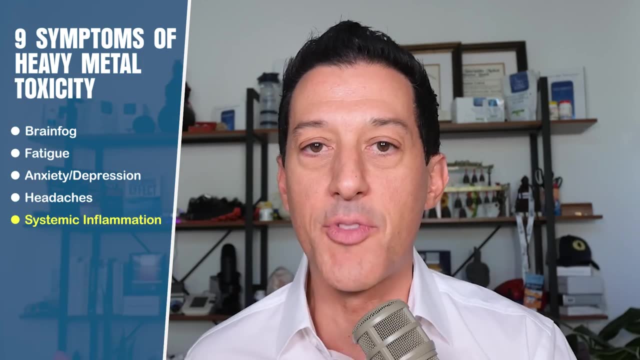 or migraines. The fifth one is systemic inflammation. So the systemic inflammation that we just spoke about before means whole body, systemic, It's everywhere. right, It's the entire system of the body. Well, what does that often look like? For many people it looks like allergies, or it looks 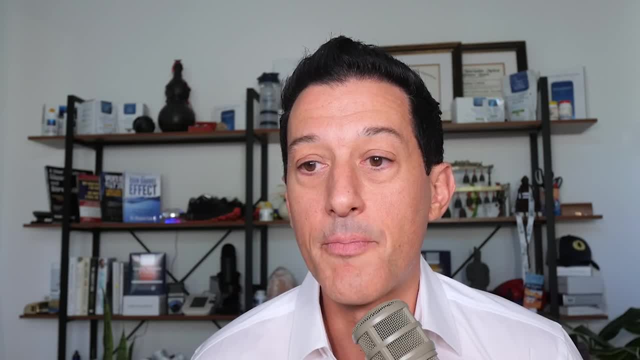 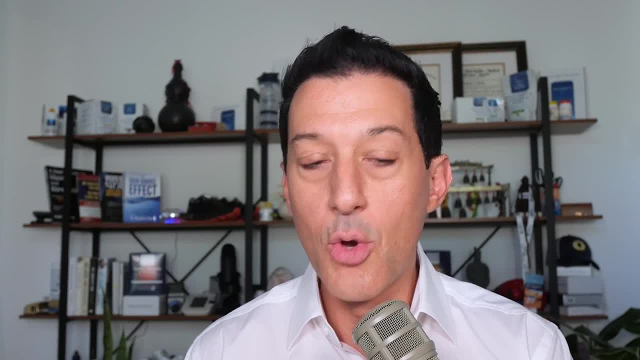 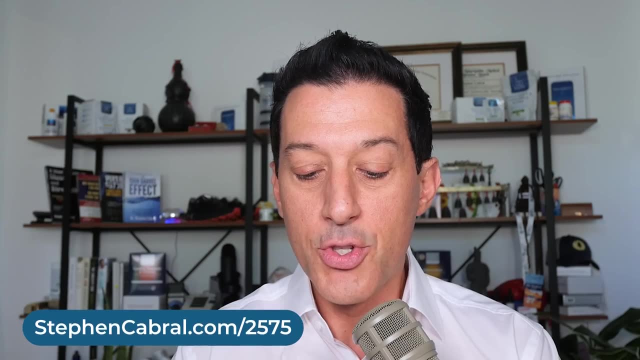 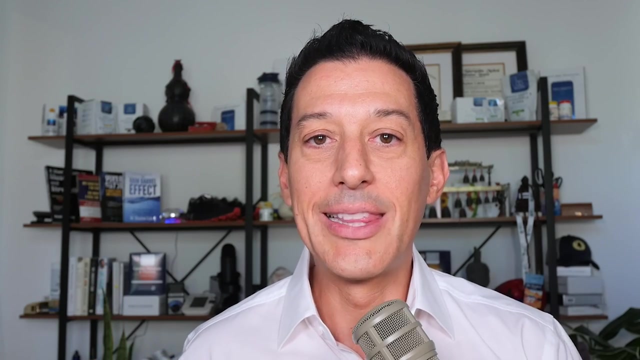 If you don't know what stealth pathogens are, we will link up that podcast for you too, and that will be at stephencabralcom forward slash 2575.. So what I want to share with you on that as well is that systemic inflammation also leads to the breakdown of your genetic weakness. right So for. 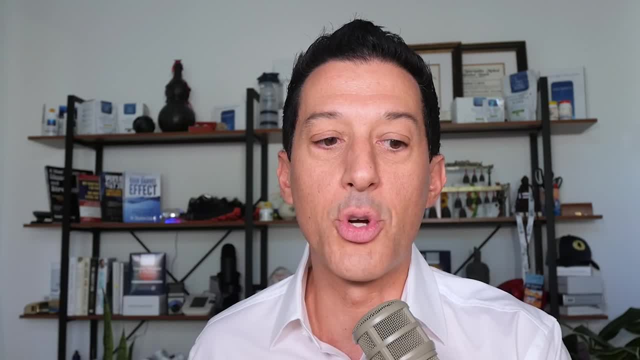 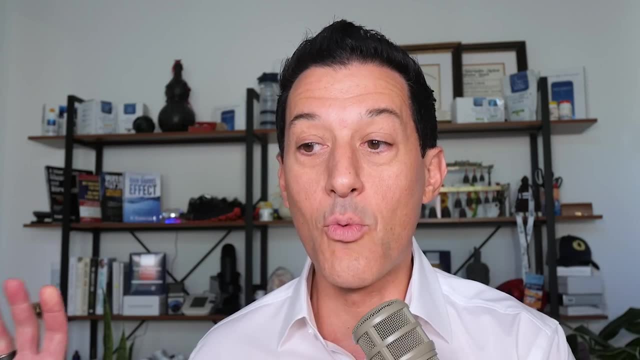 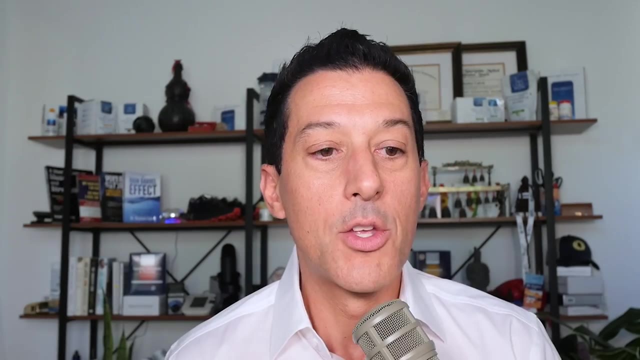 example, in my family it's an autoimmune issue called rheumatoid arthritis, which I want to get to towards the end, But always remember that inflammation goes to that already traumatized area, so like with an injury, or the weak area that you're susceptible to. So the next one is: 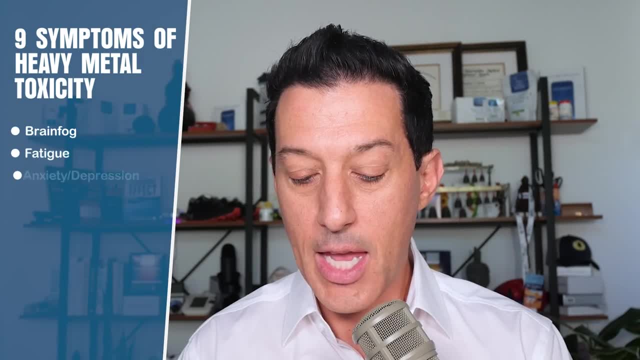 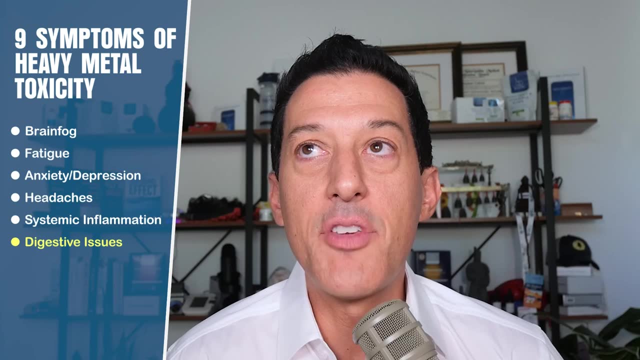 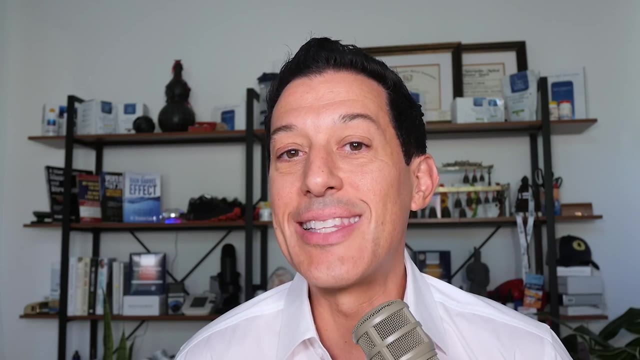 going to be digestive issues and bloating And with digestive issues and bloating, the reason why this is so important is that many times, the heavy metals which cause inflammation in the gut, which leads to then intestinal permeability, which then leads 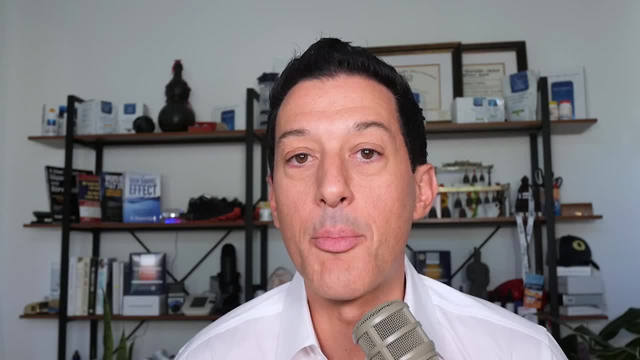 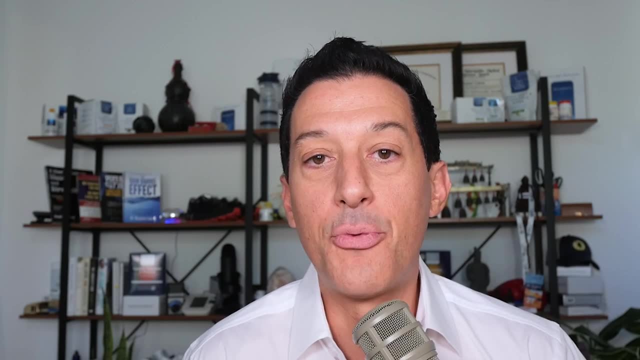 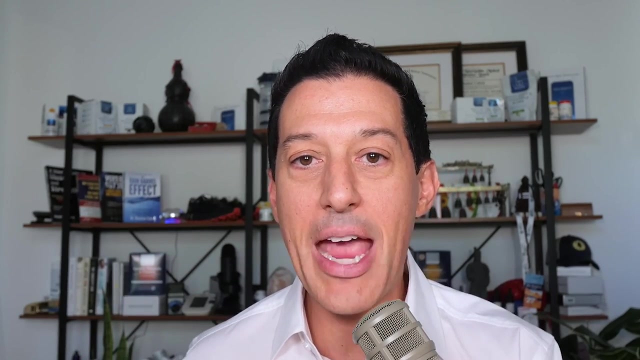 to an exacerbation of the immune system, which we're going to talk about in number nine Now. before that happens, though, there can also be a buildup of biofilms, And biofilms are a gel-like and fibrin-like structure that helps protect the parasites, the yeast and the bacteria that may be. 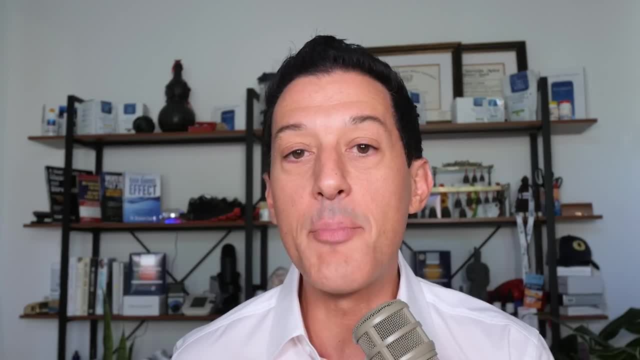 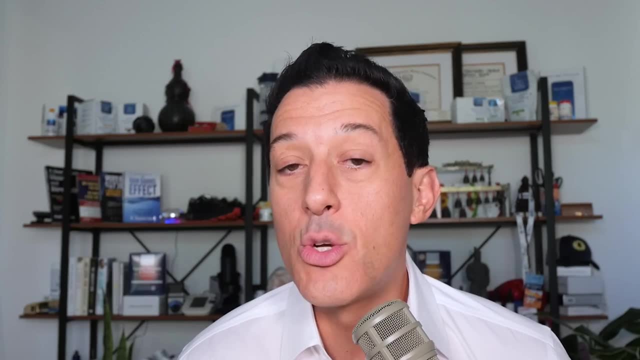 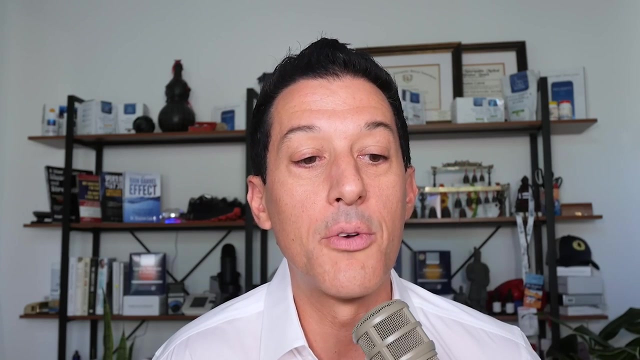 growing and living below them. Now, heavy metals are quite useful for biofilms because they add more rigidity to them. This is why, whenever we do a heavy metal protocol, we do like to include those biofilm disruptors. The one that we use is called flora film. Number seven is chronic pain. Many people dealing with chronic 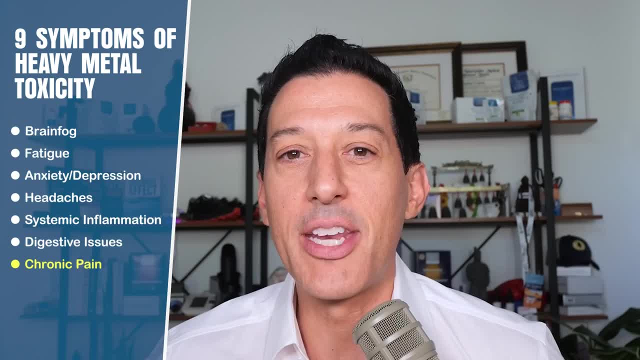 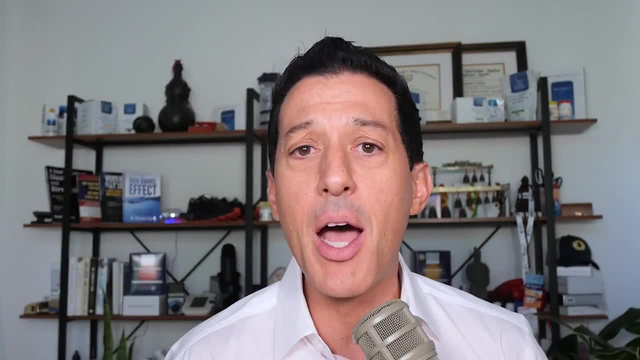 pain and putting this cause into something else, like: oh, I had an injury, I'm getting older, I'm sleeping in the wrong bed. whatever it might be, Keep in mind that heavy metals that create inflammation, which they pretty much all do, could be one of the sources. 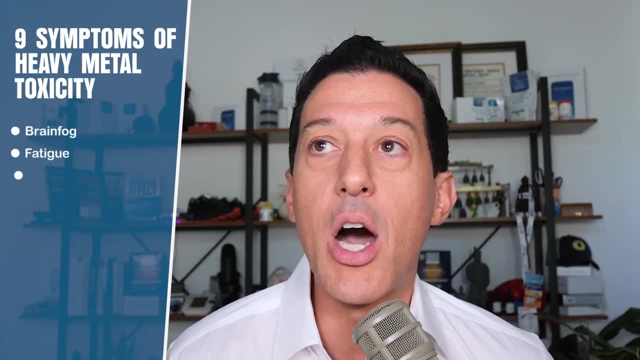 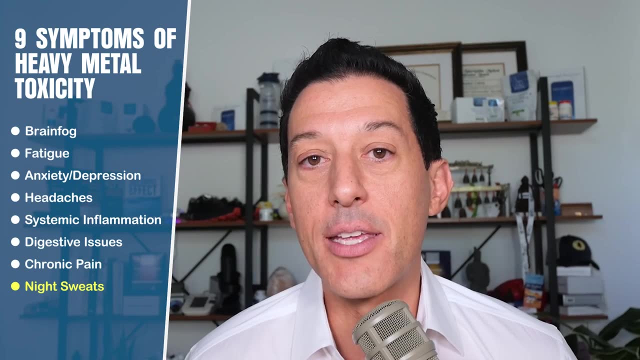 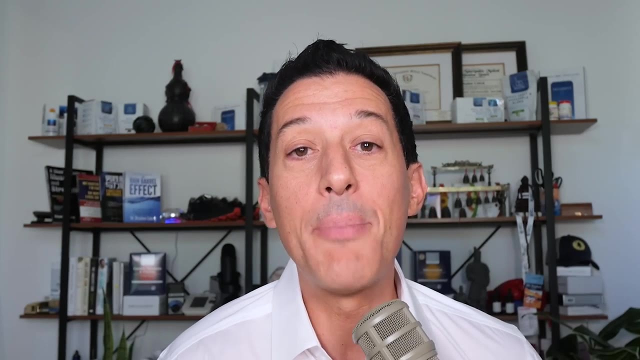 of your chronic pain. Number eight is night sweats. So often we blame night sweats on hormonal-based issues, and many times that is absolutely the case. But if you check for hormonal issues, if you check for parasites, it very well may be heavy metals. And number nine is this: 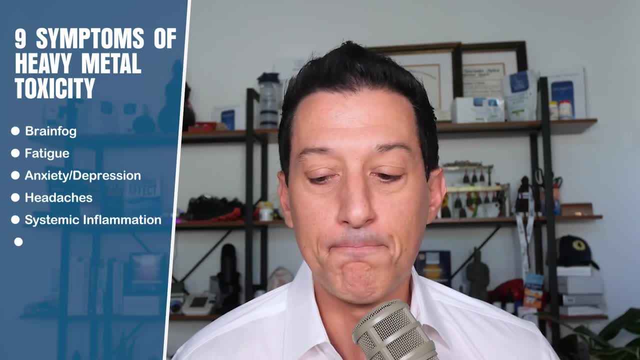 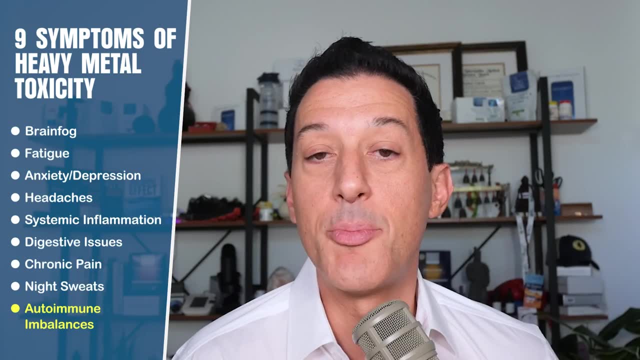 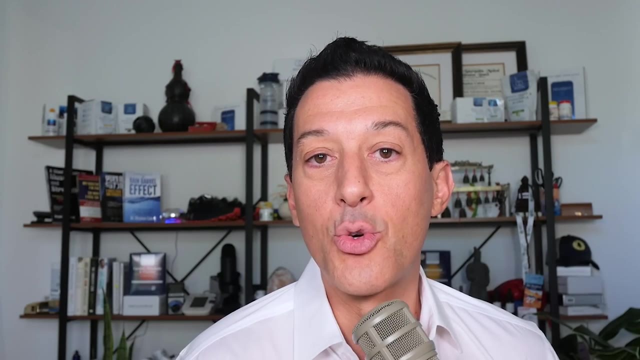 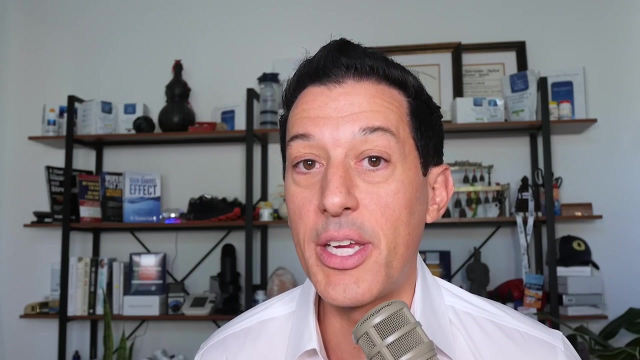 autoimmune imbalances. Think about this: By taking in too much mercury, you may be affecting your thyroid and Hashimoto's thyroiditis. How could that possibly be Well, when you are taking in what's called a halloid group metal? those metals could be things like bromine or bromides. It could be things like chlorine. from water or vapors gas. It could be from mercury as well. There are others, but those are the main ones. Whenever you take those in, you're displacing iodine, And you need iodine in order to make thyroid hormone. Without it, you're not making enough hormone. You can obviously medicate yourself through that, but why not find the underlying root cause? But the other thing that mercury can do is can actually cause inflammation in the thyroid in an immune system attack on the thyroid due to. 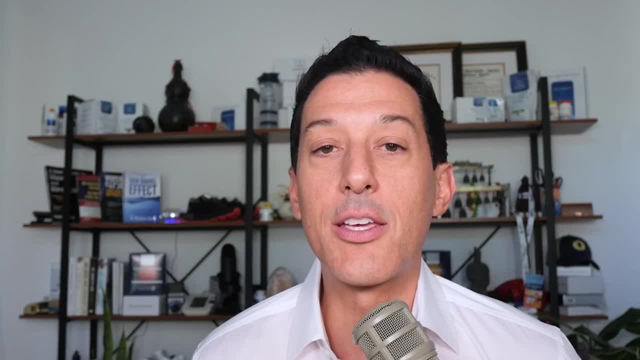 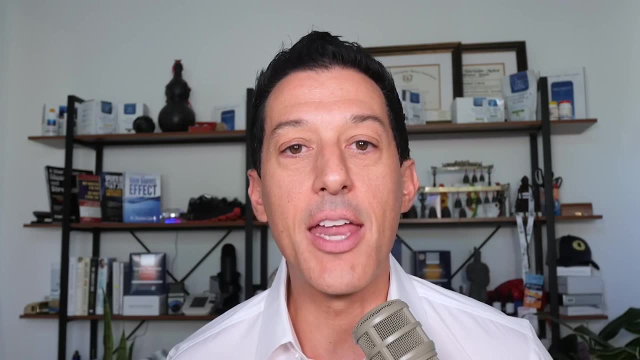 potentially mercury in the tissues. So please do not take an endocrinologist's one-sided viewpoint of saying oh, it's just genetic and leave it at that. I always recommend getting to the underlying root cause. If you didn't have Hashimoto's at, five years old. why do you have it at 15 or 25 or 35?? I know you might have a genetic predisposition to it, just like I do to a rheumatoid arthritis, but it does not mean that you have to have it. 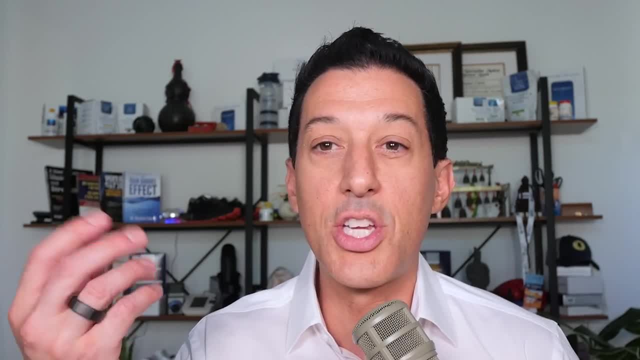 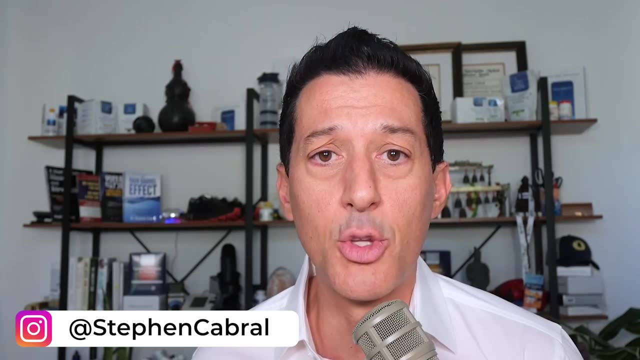 So my recommendation is that we check for heavy metals, because maybe they end up in the tissues of the joints and we get RA. Maybe they end up in the nervous system and we get MS. Maybe they end up in other organs and we get lupus right. So what I want us to do is always: 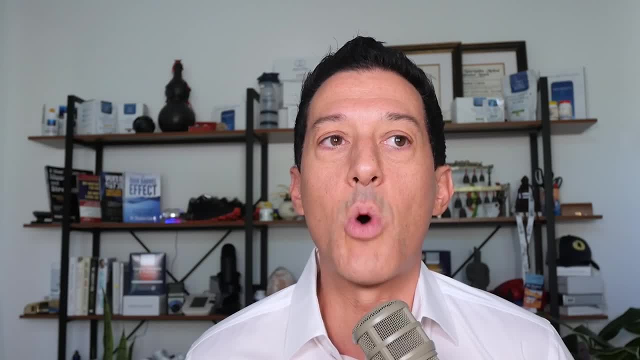 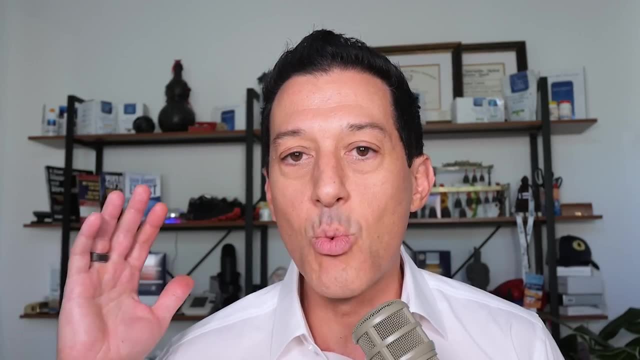 ask why. Why do I have an autoimmune issue? Why do I have cardiovascular issues? Why do I have type 2 diabetes? Why do I have high blood pressure? Why do I have cancer? Why do I have these things? If you ask why, enough, you are going to get your answer. You really will. Now, it doesn't mean 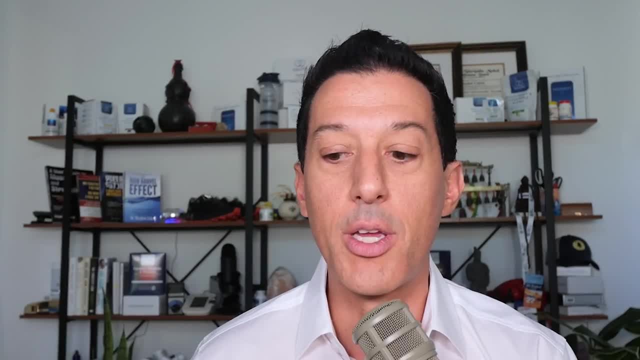 you're done. Okay, so now you have your answer. Maybe it's heavy metals, Maybe it's high levels of mercury, Maybe you ran a minerals and metals test and you found this out. Great. So now you know. What do we do? Well, we're going to do a test. We're going to do a test. We're going to do a test. 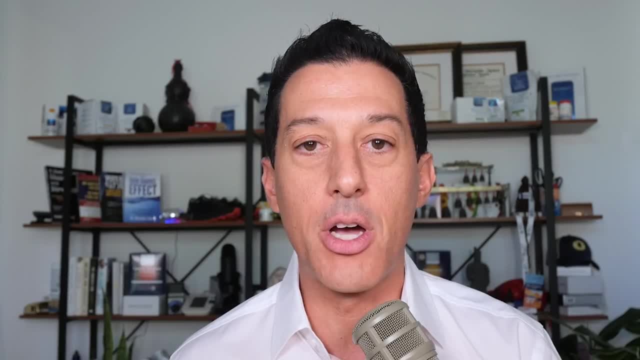 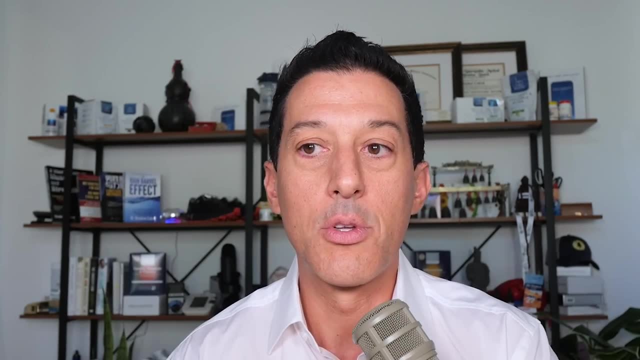 Well, after that we begin something called a heavy metal detox. Well, first I should say this: whether it's mold or parasites, eliminate the source. You know like, eliminate the source. So if you're living in a house with mold, got to get rid of the mold, right, Got to move or get. 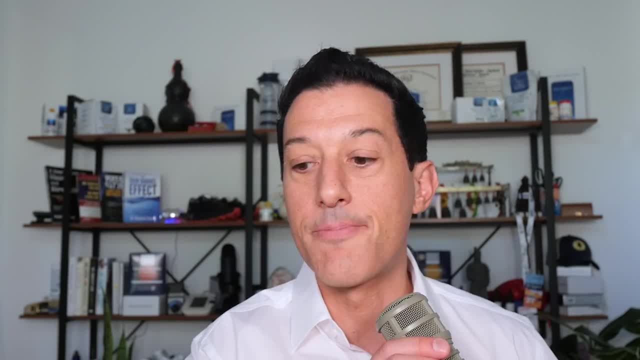 rid of the mold. That's what I did. I had mold damage in the house, Had to get rid of the mold right away. right, I'm running air filters trying to cordon off that area, but I'm getting rid of. 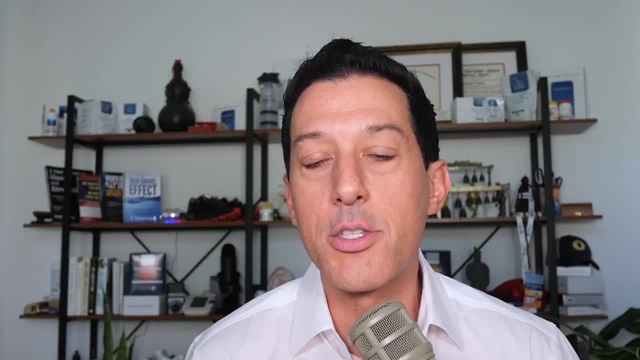 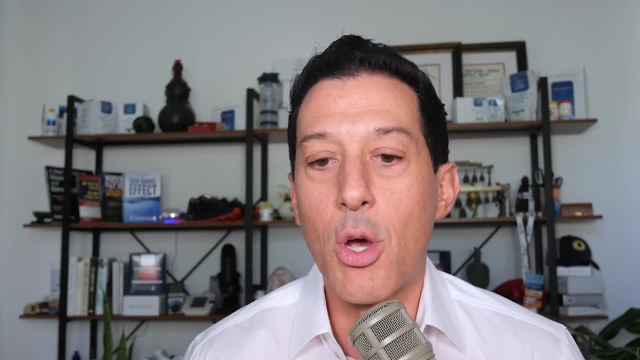 that Then I'm going to do specific protocols. Well, with the heavy metal detox, you want to make sure that you are getting rid of the mold. You want to make sure that you are getting rid of the metals from your body as well as not putting more in. So a good functional medicine detox to 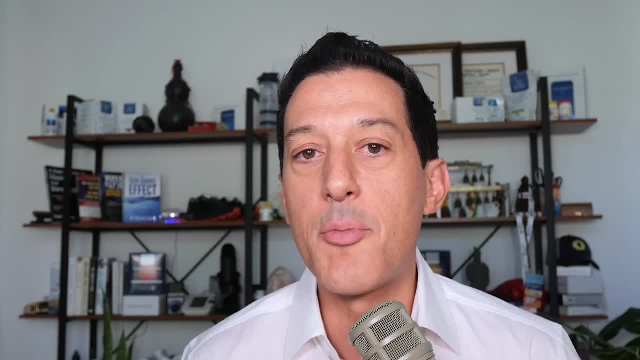 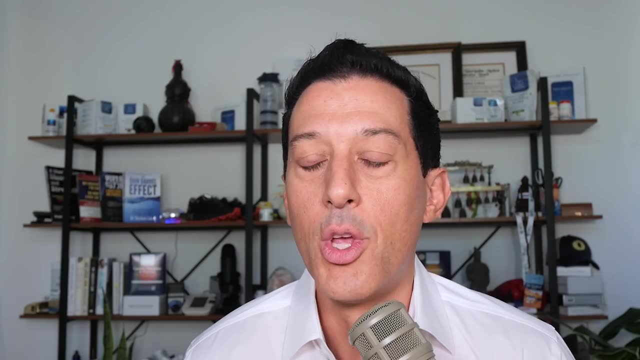 open up those liver and drainage pathways and then you're going into a heavy metal detox. Make sure that it contains things like craxel, chlorella or chlorella. Make sure it contains things like cilantro. You want vitamin C in there. You want probably a good binder that contains 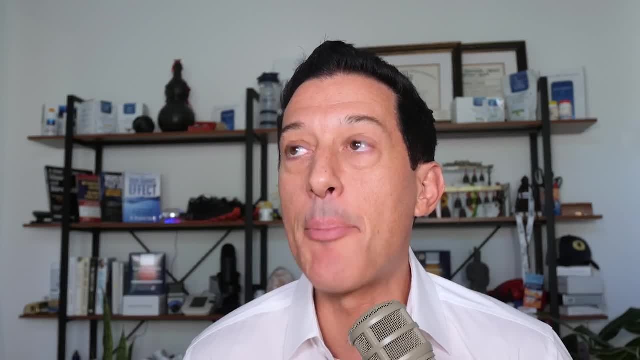 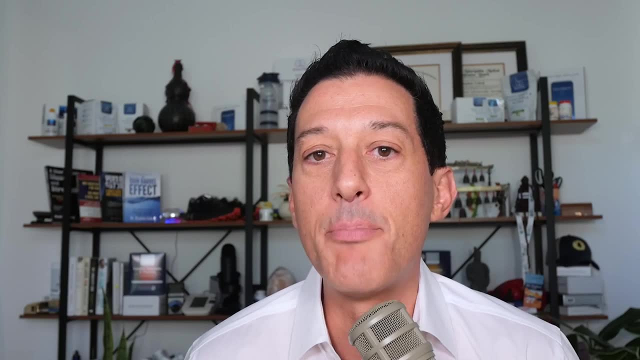 things such as bentonite, clay and apple pectin is a really great one, Humic acid, fulvic acid. Another really big one is silica Or bamboo shoots, because that'll bind to metal. So you want those things in order to be able to. 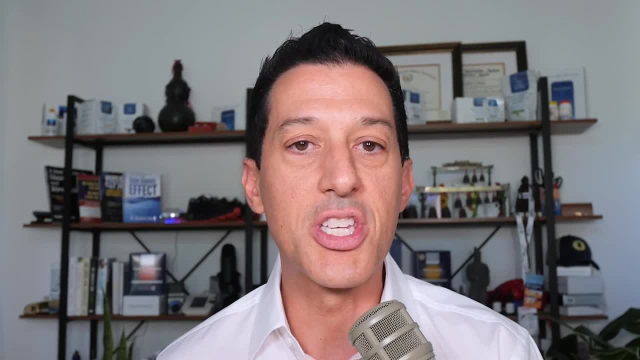 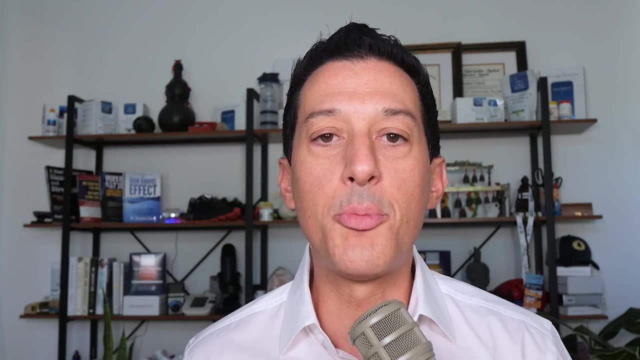 pull these things out of your body before the accumulation just continues and continues over years, Because, as I was saying earlier, disease does not happen overnight. Disease is an accumulation, a filling up of the rain barrel, And as the rain barrel fills up and it gets towards the top, 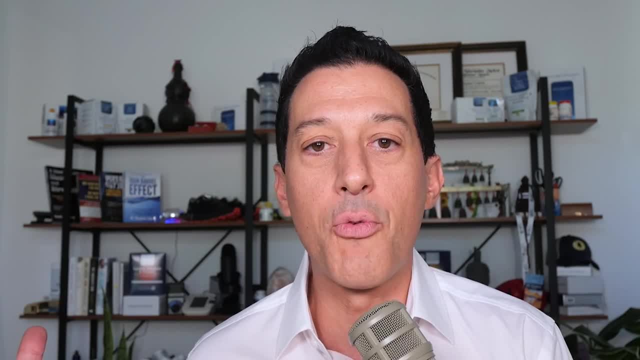 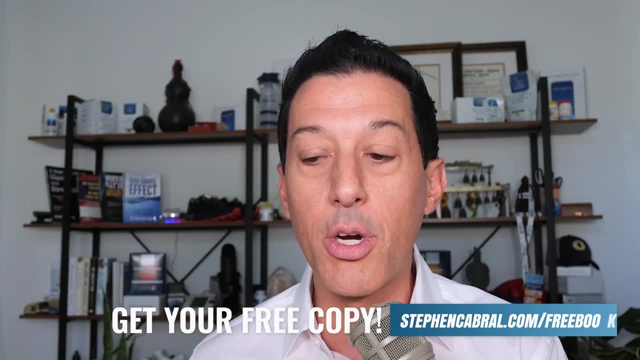 we feel the symptoms, We feel more and more symptoms And then all of a sudden it overflows, and that's when we get our diagnosis. Now can you empty the rain barrel at any time? Yes, you can. Is it easier to empty the rain barrel earlier? 100% right, Because you have more to give It's. just easier. You're not overwhelmed with all these symptoms like brain fog and fatigue and anxiety and depression and headaches and allergies, or post-nasal or low-grade asthma or digestive issues and bloating, chronic pain, night sweats and autoimmune issues. So hopefully today's show. 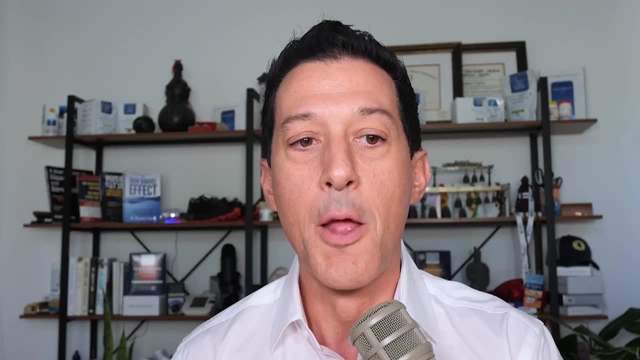 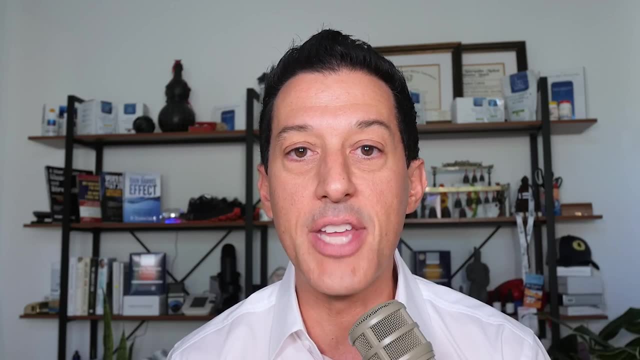 was helpful. Please let me know how I can help. I'm happy to do follow-up shows, But I wanted to get this information to you see if it connected with you. You can run a lab right at home called the Minerals and Metals Test- simple hair sample to look for those metals. 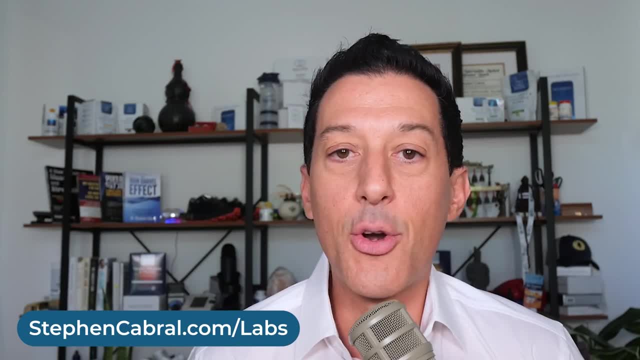 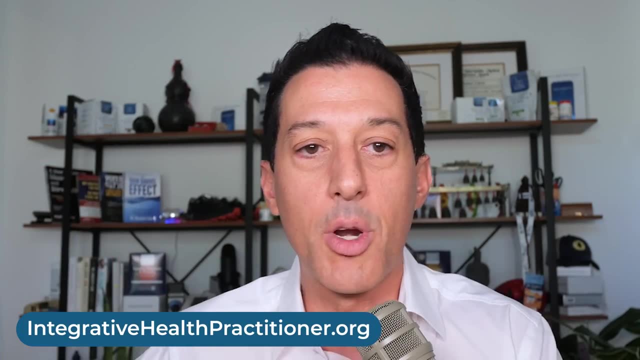 That's at stephencabralcom. forward slash labs or head on over to integrativehealthpractitionerorg. Find an integrative health practitioner- a level two, anywhere in the world. You can work with them, because I want to make sure that you know that you can work with anybody to get these labs. 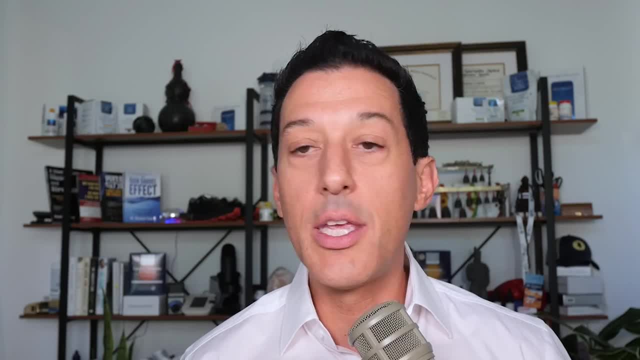 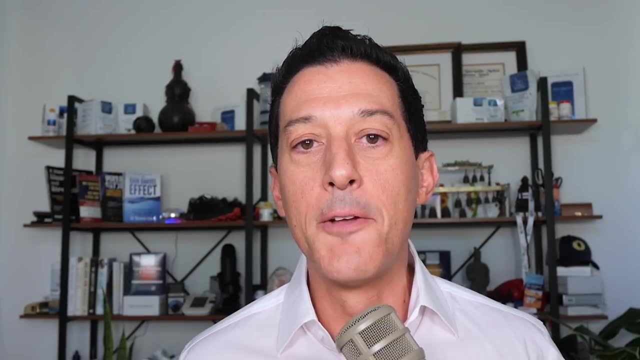 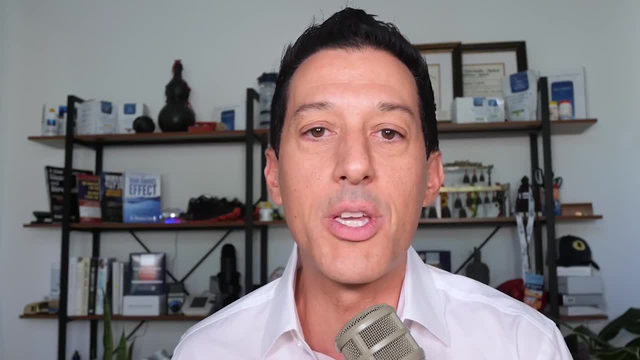 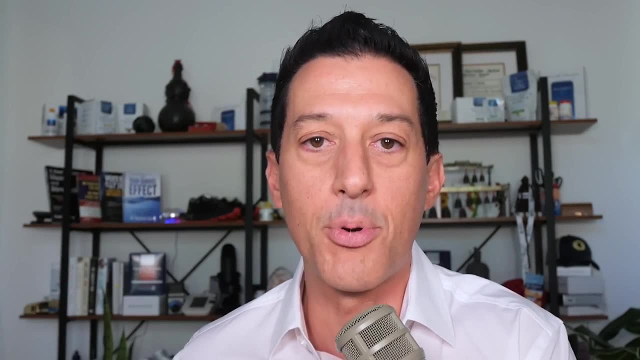 every day, And just because I know that chemicals and heavy metals are ubiquitous in the world that we live in. And so if I know that, then I'm just going to gradually just keep emptying that rain barrel on a yearly basis, just like I do. a parasite protocol, So same thing for all the 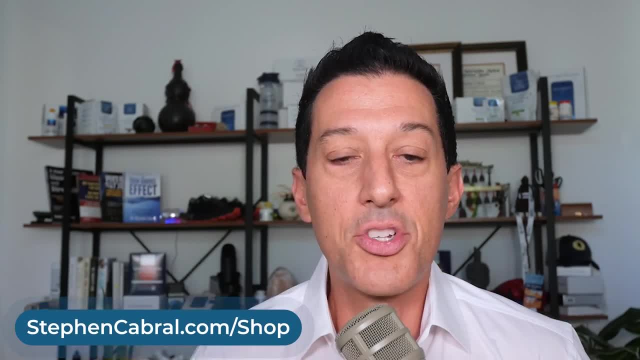 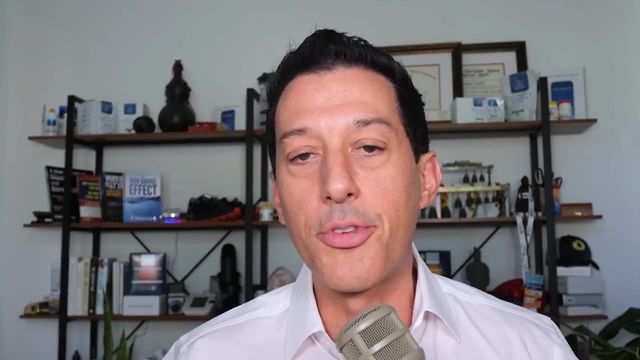 protocols. You can find those at stephencabralcom forward slash shop. Just type in heavy metal and you'll find it, or para pro and you'll find that parasite one and CBO for digestive- You'll find all the protocols. They're all open source. We share with you all the ingredients in them. 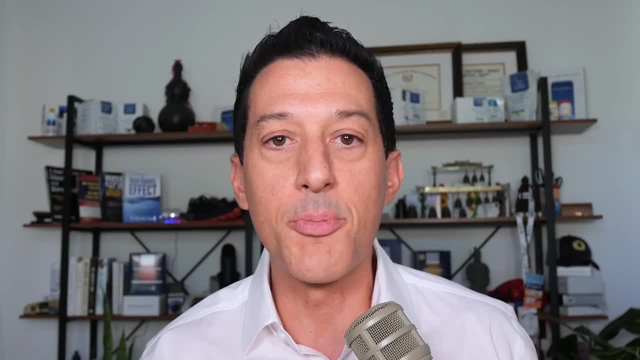 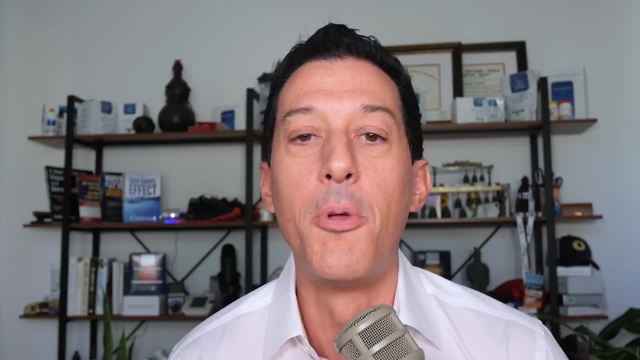 So again, just let us know how we can help. This is a true functional medicine practice. We've been working with people for many, many years- well over a quarter of a million appointments- And we, just again, we know what works. We want to be able to help. So